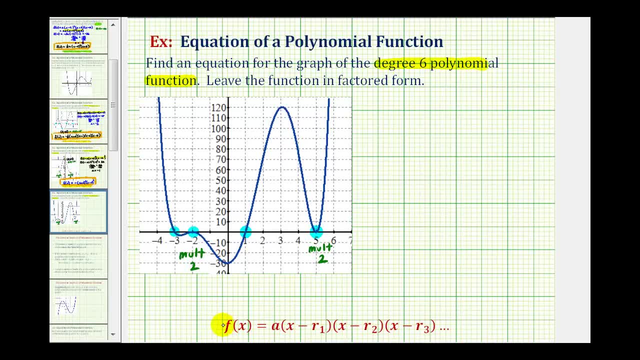 To do this we'll use the factored form of a polynomial, Given here below, Where a is a constant and r sub one, r sub two, r sub three and so on are the roots, or zeros of the polynomial function. But to determine the value of a we'll also have to identify one more point on the function. 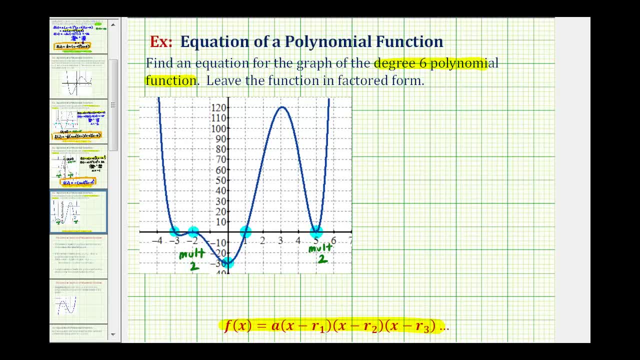 Let's go ahead and use the y-intercept or this point here, Where the coordinates are zero, negative thirty. So we'll first find the factors based upon our roots or zeros, And then we'll find the value of a using the point here. 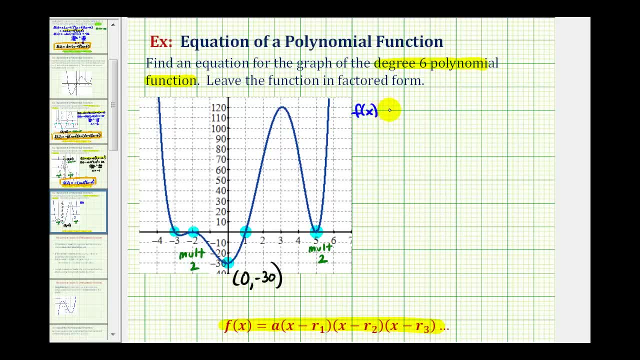 So we'll have f of x equals a times. the first zero is x equals negative three, So the factor must be x minus negative three or x plus three. The next zero is negative two, So we'd have a factor of x minus negative two or x plus two. 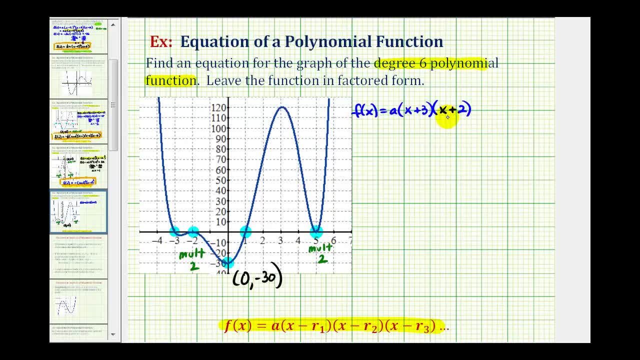 But because the multiplicity is two, We need two factors of x plus two, Or the quantity x plus two squared Next, we have a zero of one, So we have a factor of x minus one, And our last zero was x equals five. 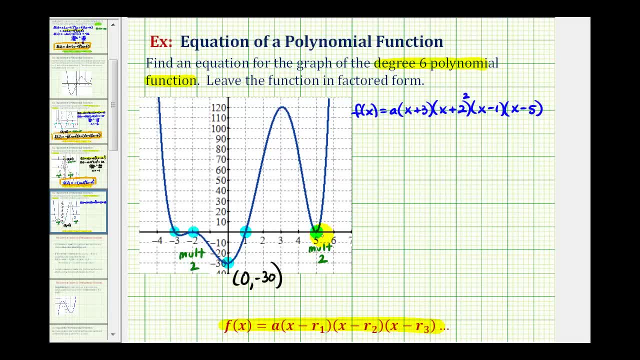 So we have a factor of x minus five, But again this has multiplicity two, So we have two factors of x minus five Or the quantity x minus five squared. So, based upon how our graph behaves, These must be factors of our polynomial function. 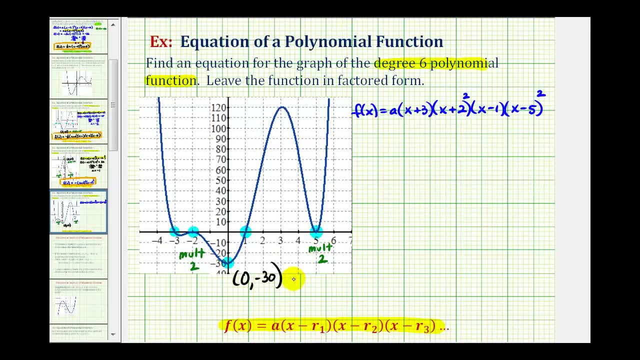 And now because the graph contains the point zero negative thirty. That means f of zero must equal negative thirty. So now we'll substitute zero for x And set the function value equal to negative thirty, Which will allow us to solve for a. So f of zero would be equal to a times. 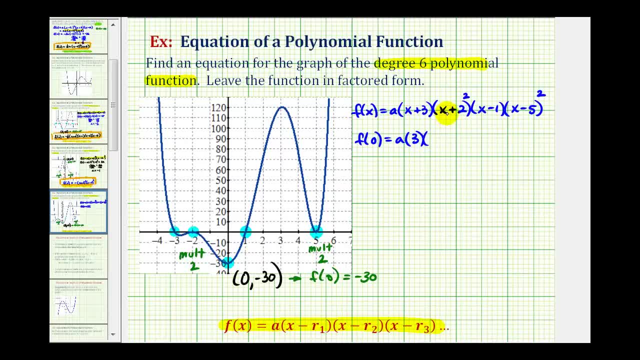 If x is zero, we'd have three here. If x is zero, here we'd have two squared. If x is zero, here we'd have negative one, And here we'd have negative five squared, And this must equal negative thirty. So now we'll go ahead and simplify this and solve for a.